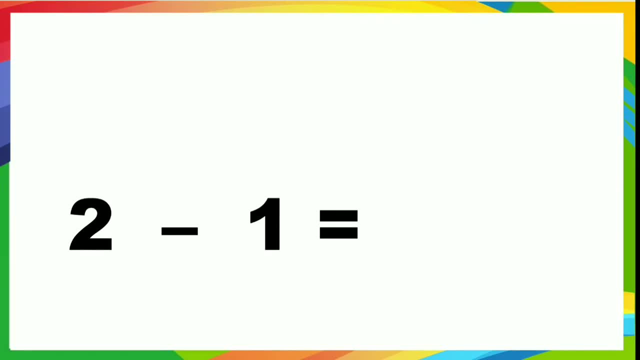 2 minus 1.. What are these Lollipops? Yes, How many lollipops are there? Two, Two lollipops are there. So if you have two lollipops and if you give one lollipop to your friend, 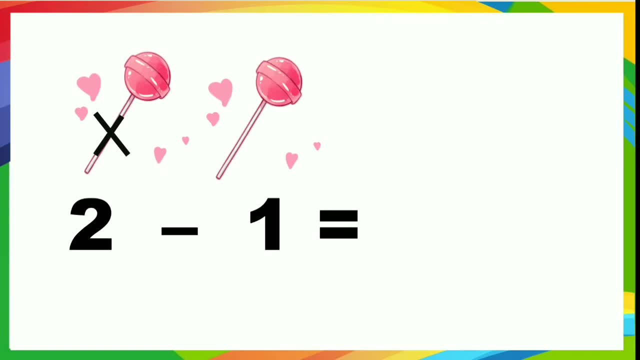 You give one lollipop to your friend. How many left with you Count children. How many left 1.. Yes, So 2 minus 1 is equal to 1.. 3 minus 1.. Hmm, What are these Ice creams? 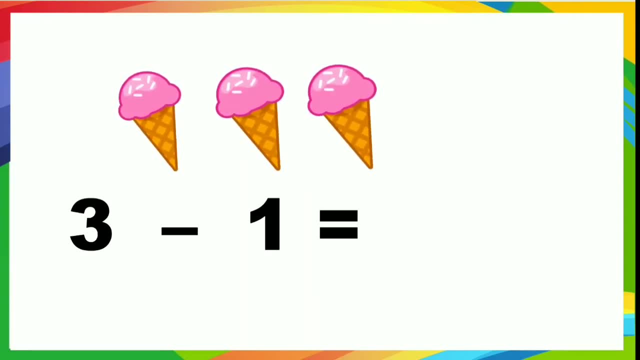 3 ice creams are there. 3 ice creams are there. If you take away one ice cream, how many left? Count 1, 2.. 3 minus 1 is equal to 2.. Okay, Now see. 4 umbrellas are there. 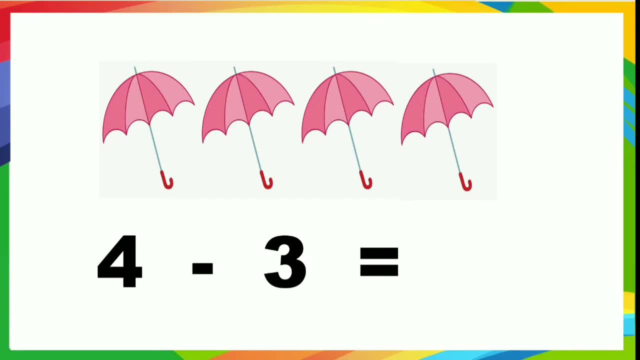 So how many you need to take away? 4 minus 3.. 3 you need to take away. Take out 3 umbrellas: 1,, 2, 3.. How many left children? How many umbrellas left? 1. Yes, 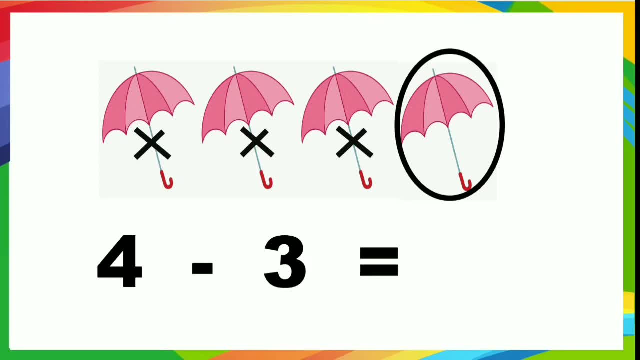 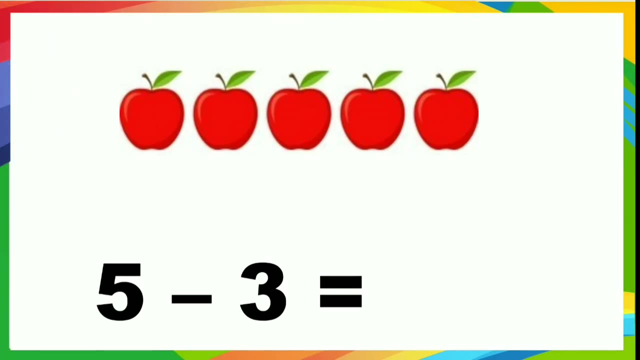 1. Yes, 4 minus 3 is equal to 1. 1. 1. 1. 1. 1.. Yes, 4 minus 3 is equal to 1.. 4 minus 3 is equal to 1.. 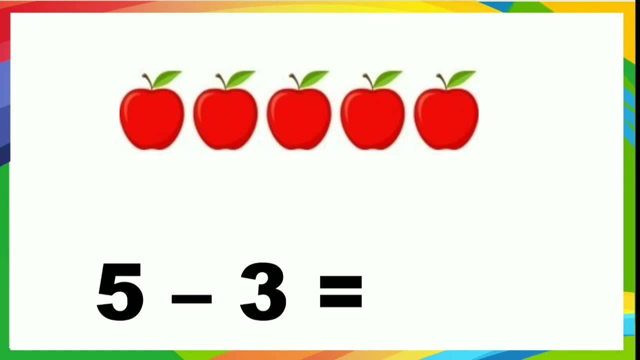 5 minus 3.. 5 apples are there. Yes, You need to take away how many? 3.. Count: You need to take away how many 3.. Count 1,, 2, 3.. How many left? 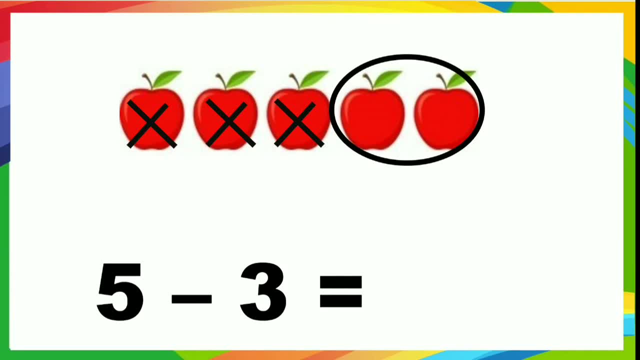 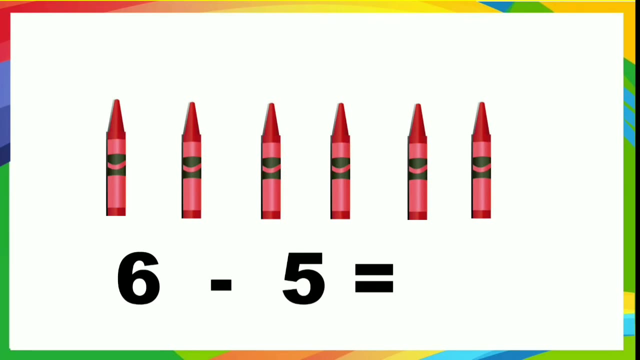 1, 2.. How many left? 2. 5 minus 3 is equal to 2. 6 minus 5.. You have 6 crayons and you need to give how many: 5.. 1,, 2,, 3,, 4, 5.. 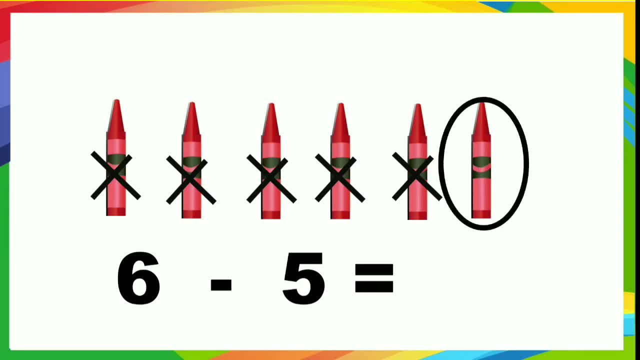 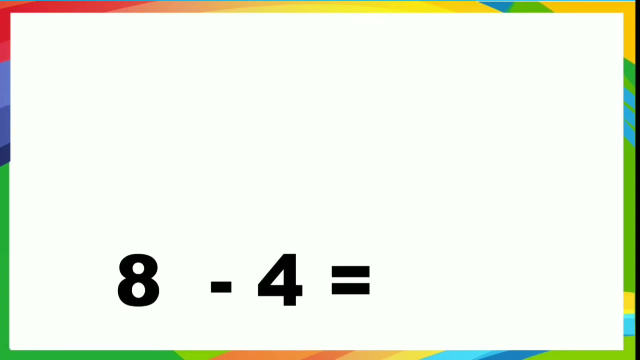 How many left children Count? 1, yes, 6 minus 5 is equal to 1.. 8 minus 4.. Let's learn with balls. Let's count 8 balls: 1,, 2,, 3,, 4,, 5,, 6,, 7,, 8.. 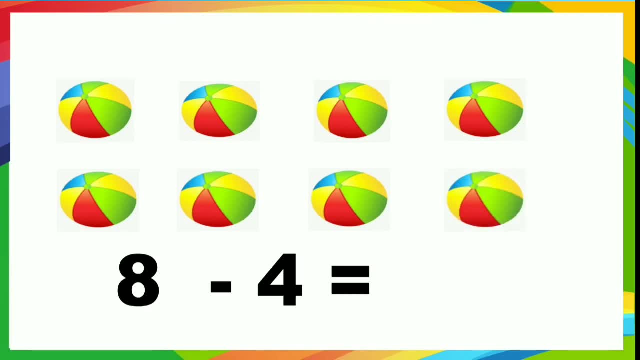 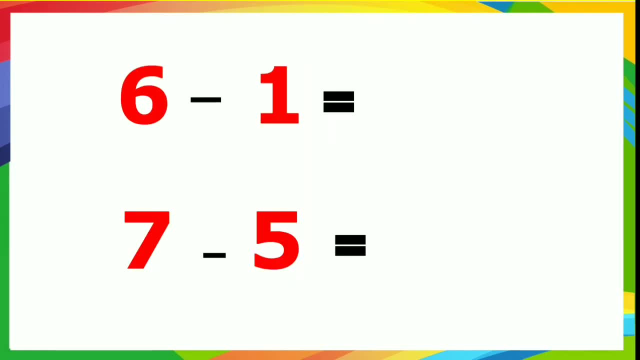 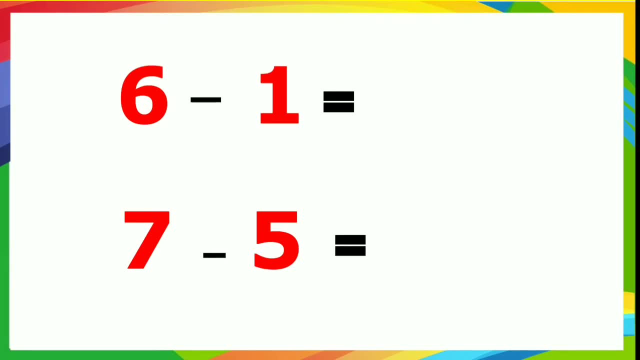 8. 8. 8. 6 minus 1.. Draw 6 sticks Like this And you need to take away how many 1.. How many left? Count? Count 5, yes, correct, 6 minus 1 is equal to 5..